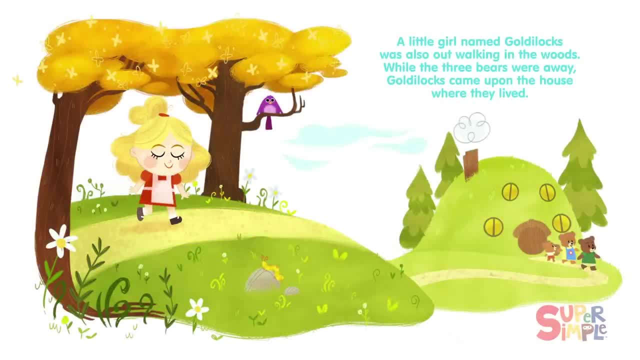 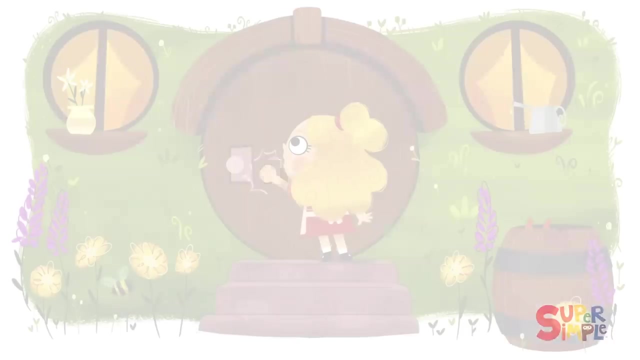 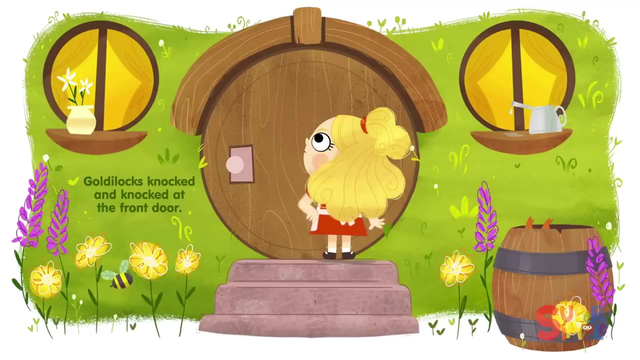 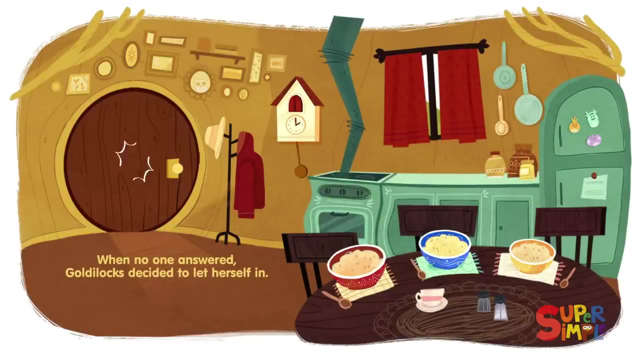 A little girl named Goldilocks was also out walking in the woods. While the three bears were away, Goldilocks came upon the house where they lived. Goldilocks knocked and knocked at the front door. When no one answered, Goldilocks decided to let her go. 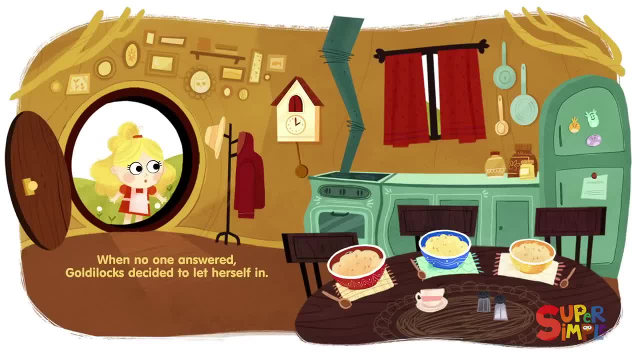 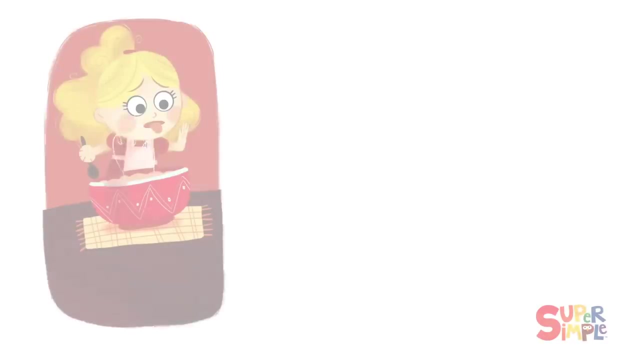 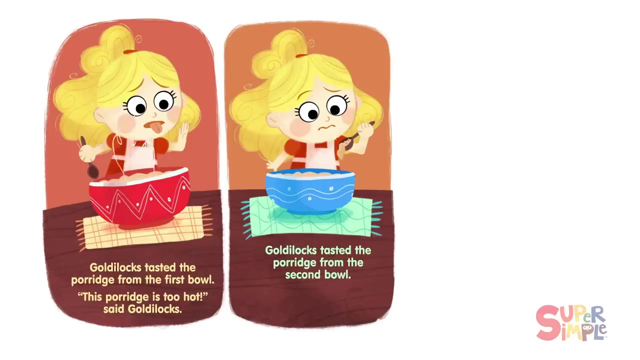 She locked herself in. She saw three bowls of porridge on the table And her tummy rumbled. Goldilocks tasted the porridge from the first bowl. This porridge is too hot, Said Goldilocks. Goldilocks tasted the porridge from the second bowl. 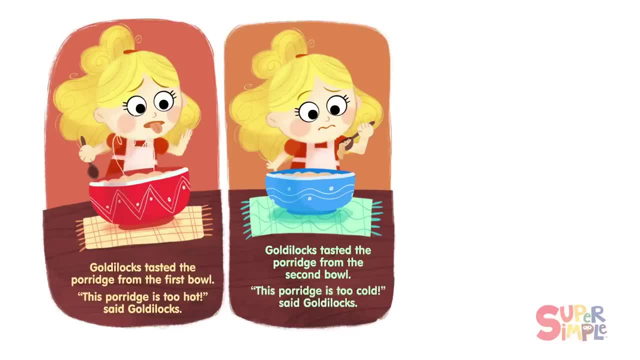 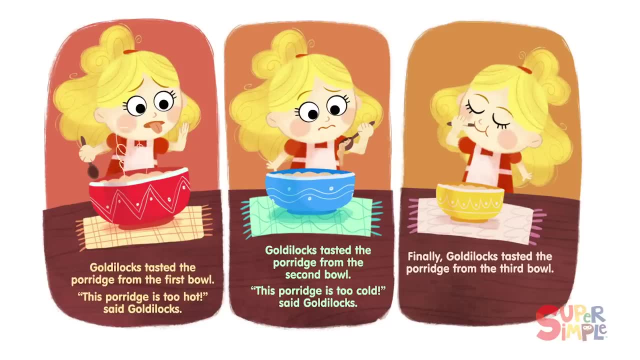 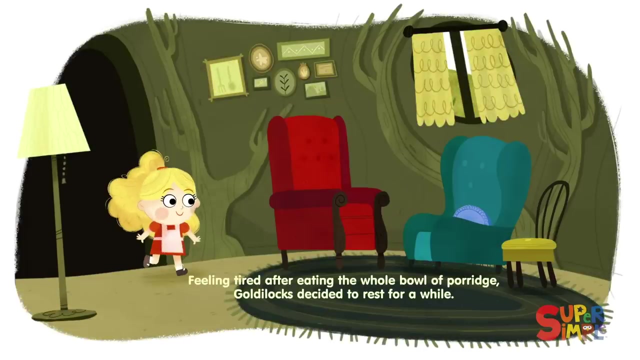 This porridge is too cold, Said Goldilocks. Finally, Goldilocks tasted the porridge from the third bowl. Ah just right, Said Goldilocks, And she ate it all up, Feeling tired after eating the whole bowl of porridge. 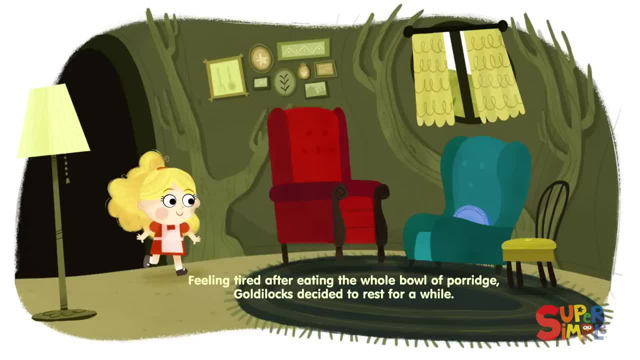 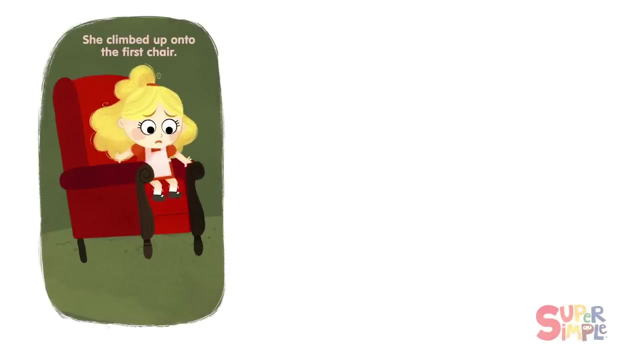 Goldilocks decided to rest for a while In the living room. she found three comfortable looking chairs. As she climbed up, she noticed the first chair. She climbed up onto the first chair. This chair is too high, said Goldilocks. 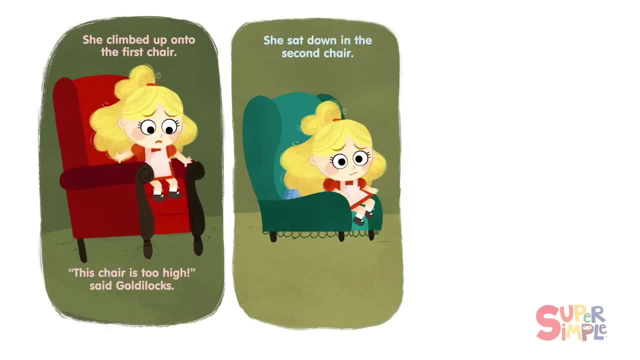 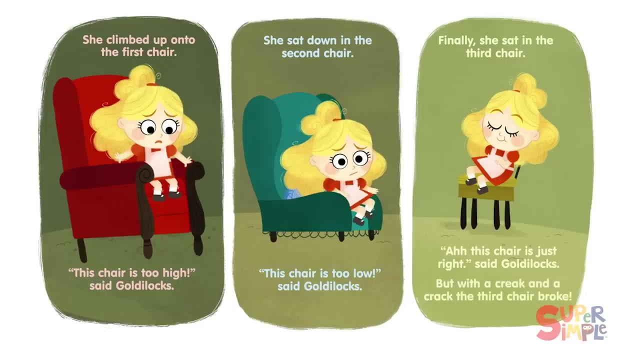 She sat down in the second chair. This chair is too low, said Goldilocks. Finally, she sat in the third chair. Ah, this chair is just right, said Goldilocks. But with a creak and a crack the third chair broke. 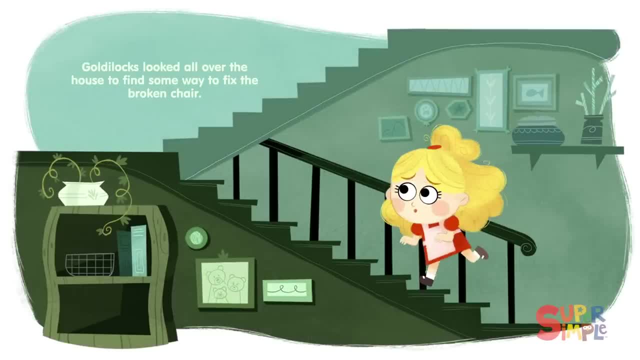 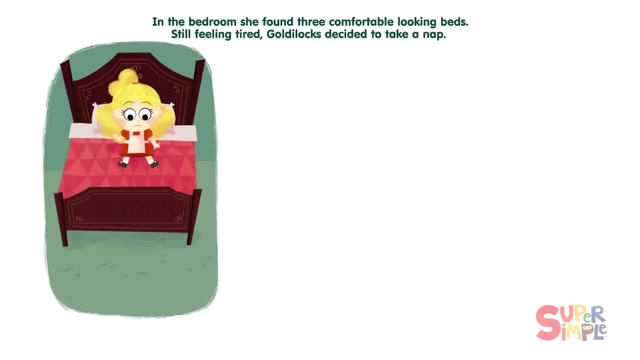 Goldilocks looked all over the house to find some way to fix the broken chair In the bedroom. she found three comfortable-looking beds. Still feeling tired, Goldilocks decided to take a nap. She laid down in the first bed. This bed is too hard, said Goldilocks. 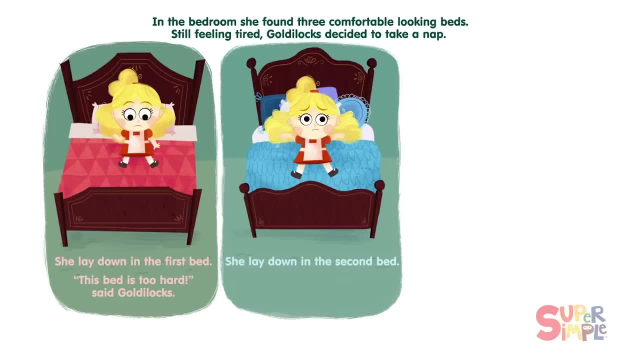 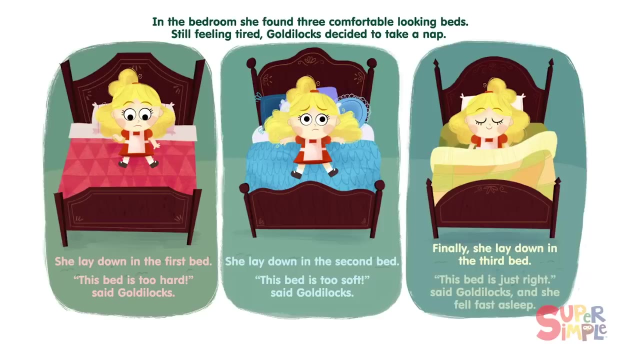 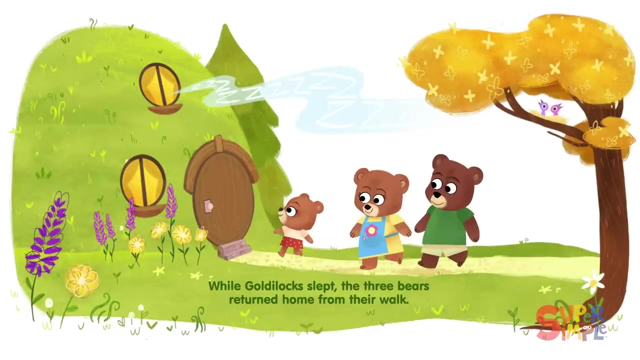 She laid down in the second bed. This bed is too soft, said Goldilocks. Finally, she laid down in the third bed. This bed is just right, said Goldilocks, And she fell fast asleep. While Goldilocks slept, the three beds were all broken. 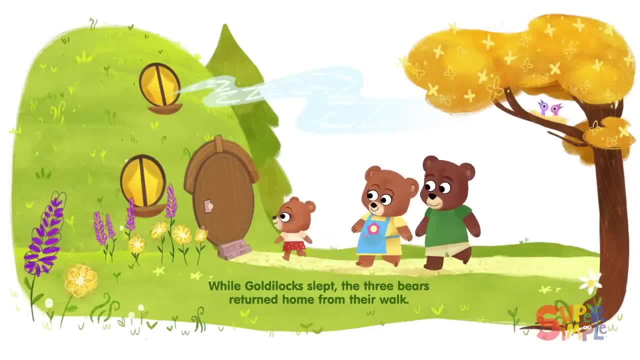 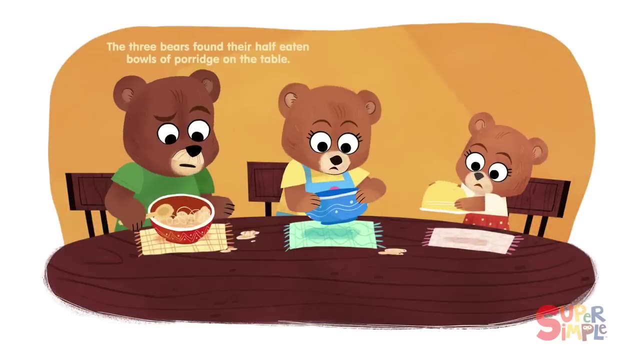 The three bears returned home from their walk. The three bears found their half-eaten bowls of porridge on the table. Someone's been eating my porridge, said Papa Bear. Someone's been eating my porridge, said Goldilocks. Someone's been eating my porridge, said Mama Bear. 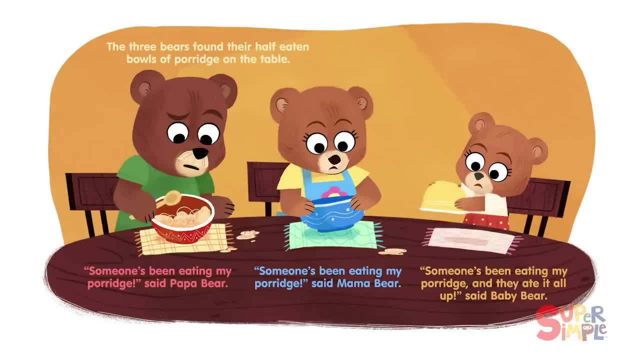 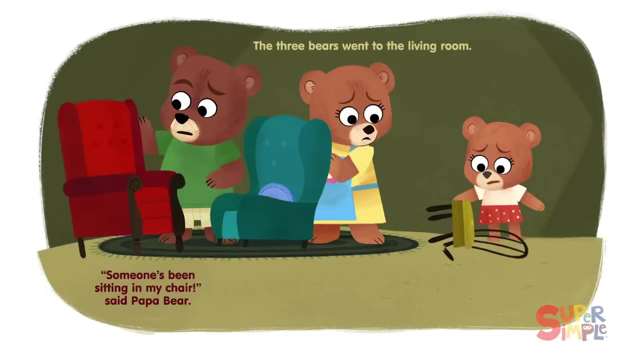 Someone's been eating my porridge and they ate it all up, said Baby Bear. The three bears went to the living room. Someone's been sitting in my chair, said Papa Bear. Someone's been sitting in my chair, said Mama Bear.